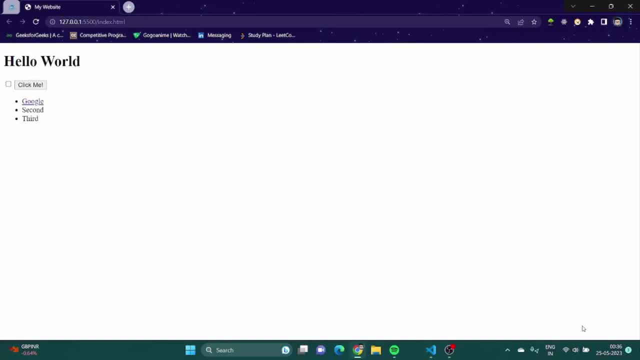 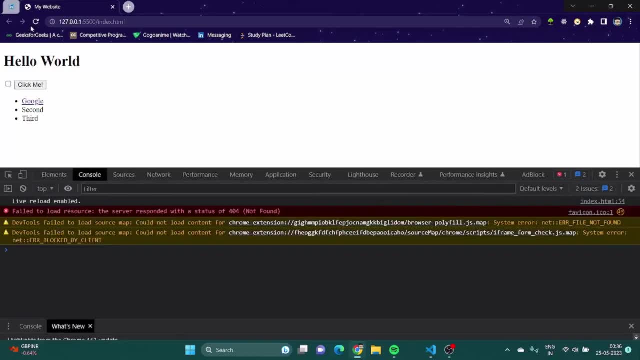 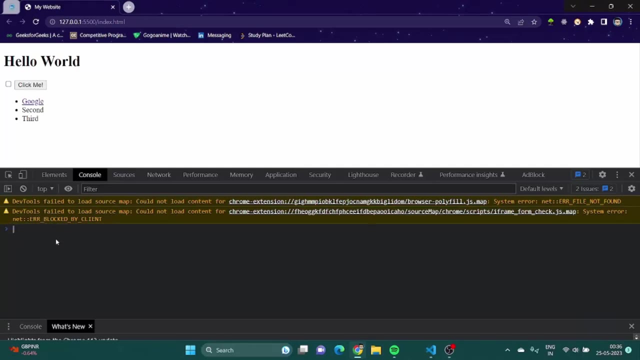 uh, let me just open it, okay. so i'll just go to more tools. i'll open my developer tools and here i am, let me just reload it and okay, great. now i have like given a few examples in the previous videos, so if i talk about them, so like, uh, you know. 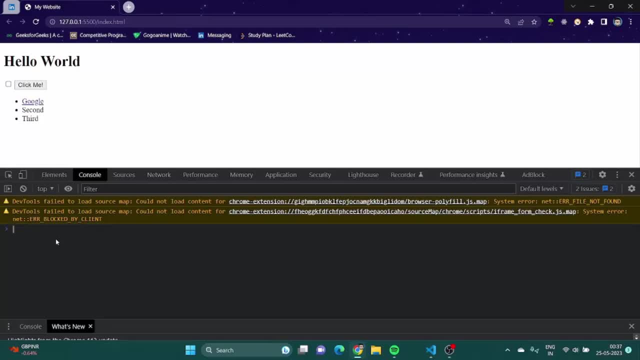 we were able to change the css style and then dynamically using javascript, by, you know, tapping into the element and then changing it using dot style. okay, so what you can do, you can simply type document dot, let's say, query selector dot. uh, first you have to query select any, which is, let's say, 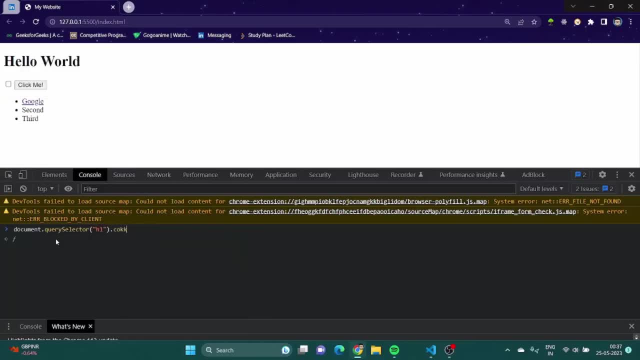 h1. right, you are going to have, let's say, style, and then we are going to have color, let's say red. so what it does? it taps into the element h1, which is this element. then it goes into its style and the style we change its color to. 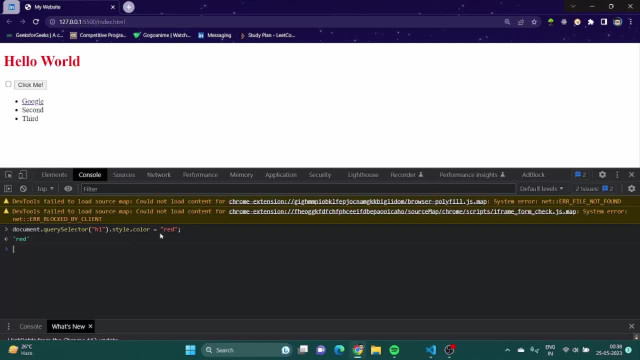 red. okay, now every single css property can be changed in this way using javascript. okay, you know, but the property names might be a bit different. as you said earlier on javascript, uh, uh, like javascript, naming conventions tend to be camel case case mean that if there is like two word word, i mean query and selector. so the first letter has 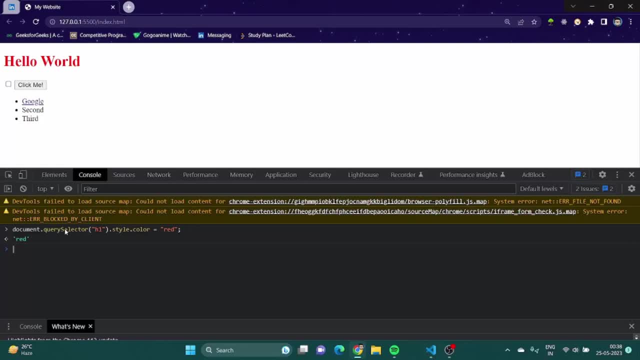 to be small case, and the second letter would be um uppercase. okay now, if you remember, there was something called uh, um, what it was like? okay, font size. so how font size was written? font size was written like font dash size as the property name in css- right, but in javascript we use it like: 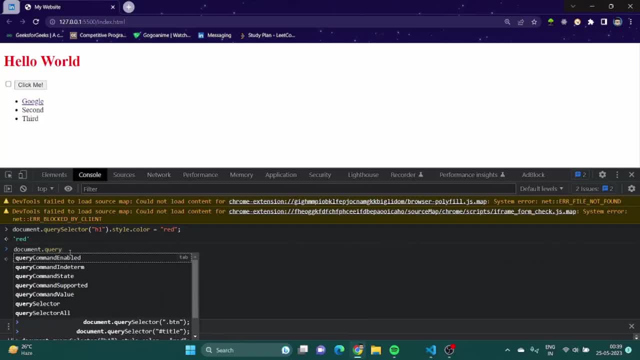 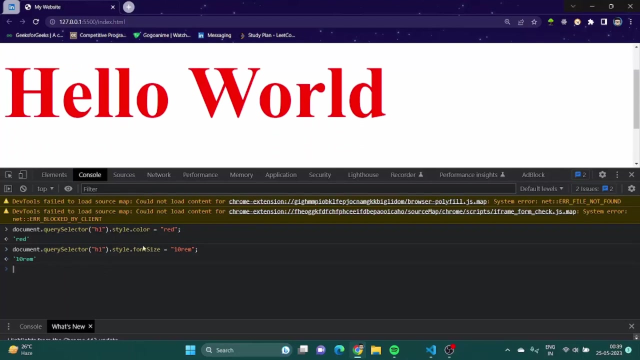 let me just say document, dot. query selector. let's say h1 dot. style, dot font size. that is how you write um. let's say, uh, any big value. let's say 10 re. okay, it is very big, but okay, you understand what i'm talking about. okay, now to have all the 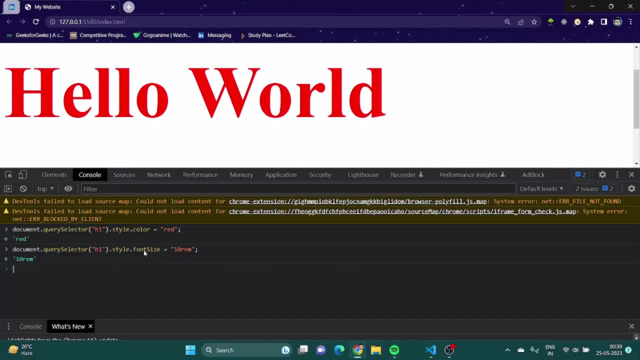 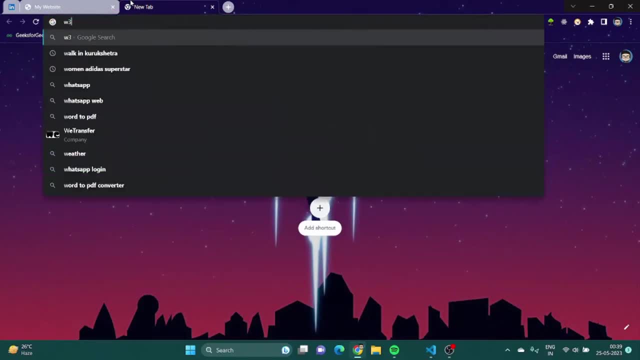 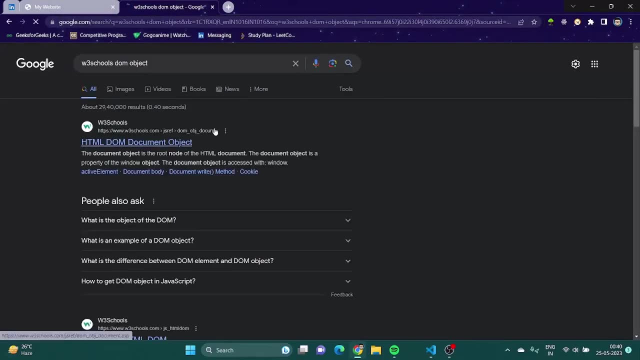 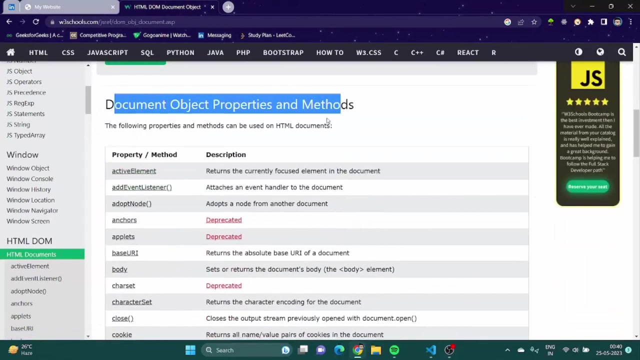 lists of you know pa. i mean css styles which you can tap into and you can change. you can go to uh w3 schools, dom object: okay, i, if i remember it was this, okay, okay, great, and here you can see all all the object properties and methods you can change. 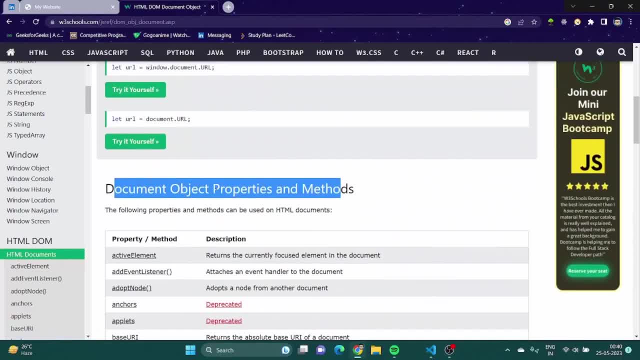 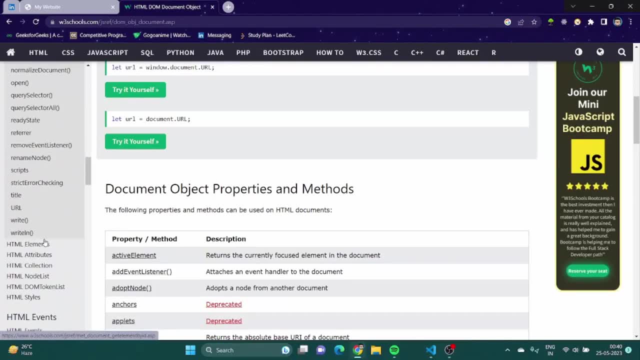 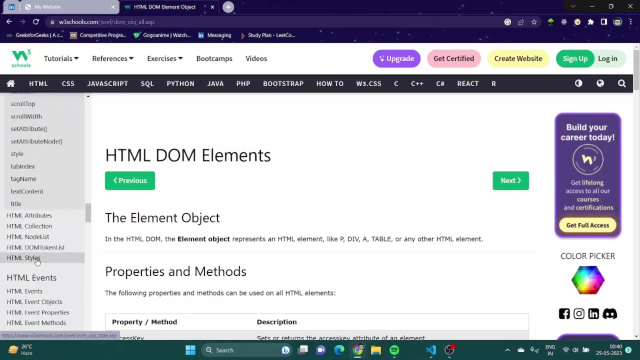 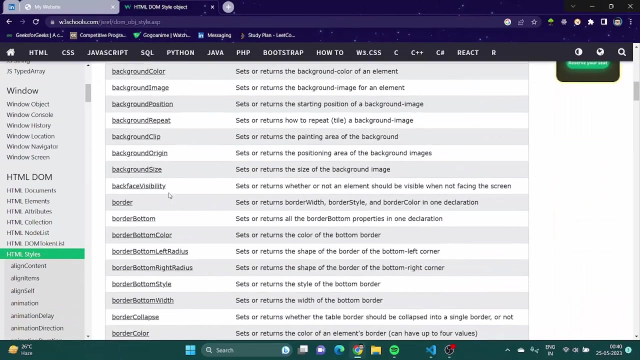 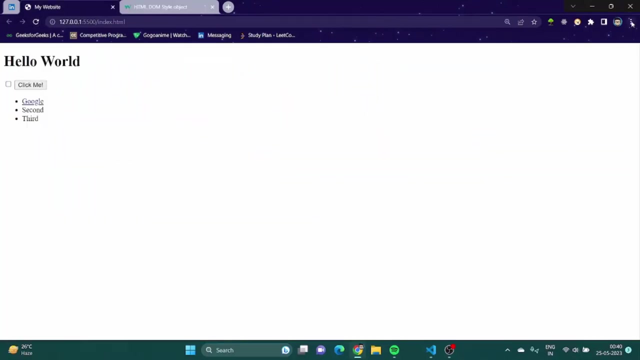 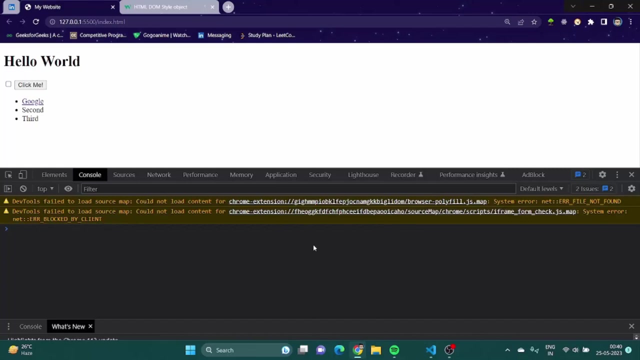 okay, uh, great, um, give me one minute, let me check. uh, which limitations do you have? so if i do something wrong in the document, switch it to: uh, um, um, i'm looking for something awesome. uh, uh, something noodles i'm going to paste and activate youtube or hello, completely obvious. 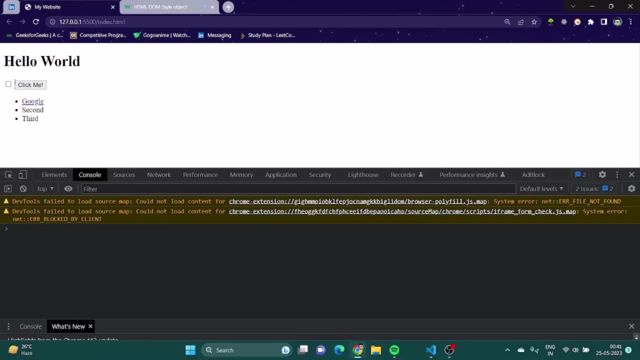 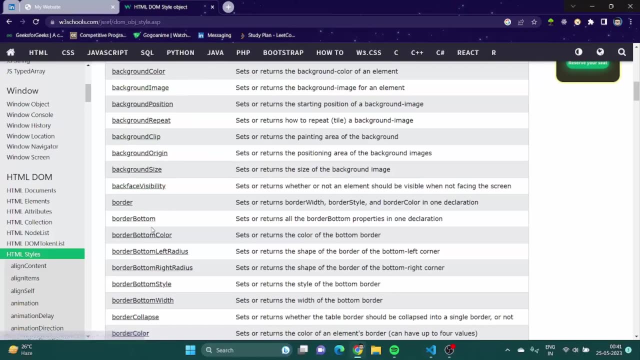 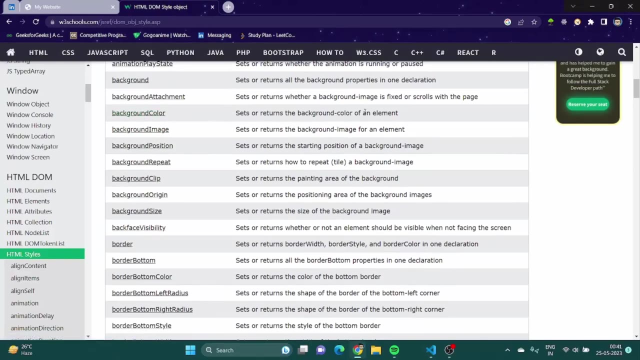 the color of this click me button. background color to yellow. so for that you need to go to Dom style object, I mean this webpage. here you can find the property name, which is you can check background color. it you know sets or it has the background color of an element. so what you will do, you will say: 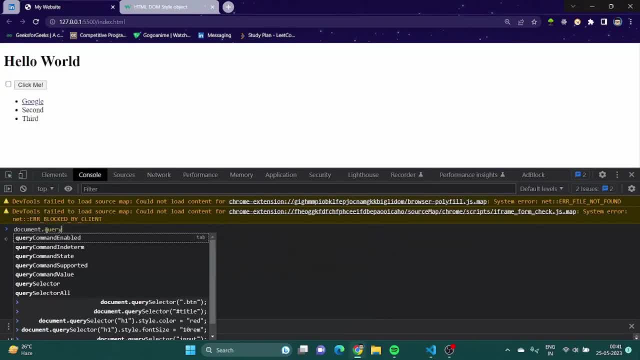 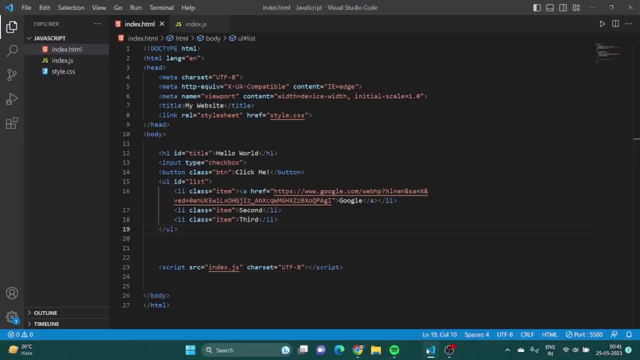 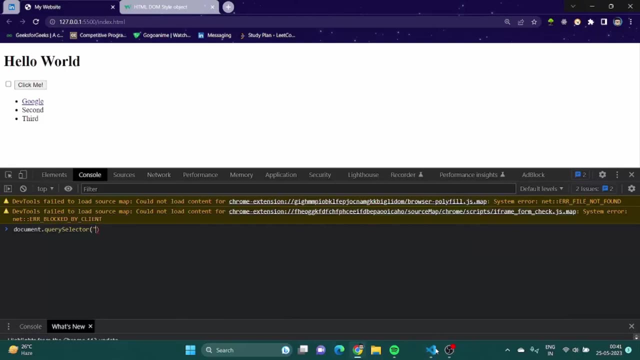 document: dot query selector. what is it? it's a button right, or you can just do dot BTN, dot BTN and this tile dot path ground color to, lets say, yellow. ok, this is done. you can see it looks nice, right, okay, great, let me just refresh it. yes, now this was one way of you know manipulating the styling of any. 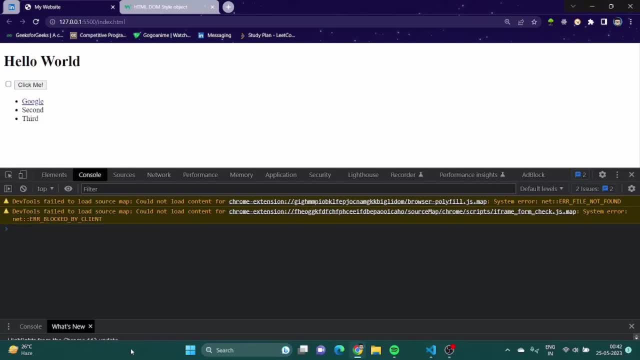 element in our page. now, the other thing which we would be talking about is how to change the content of a項 went below the content of a page, so let's change that content. so just let me an element so you know how we used to change the content. it was like document dot query selector. 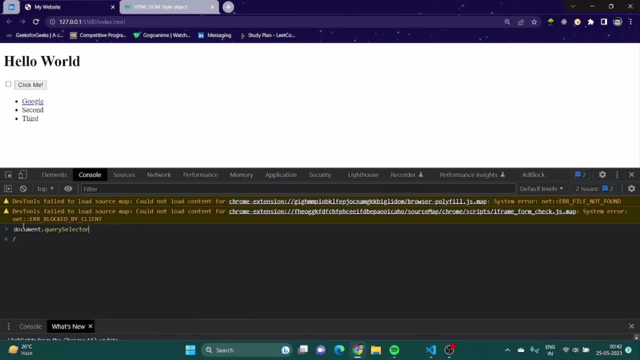 dot. uh, let's say h1 dot. inner html is equal to: let's say: bye, great. now there is another way to do it, which is uh, text content. it is like document dot, you know, we will say query selector. you will say h1 dot, you will say text content. let's say, we'll just again say it: hello, okay. now these two. 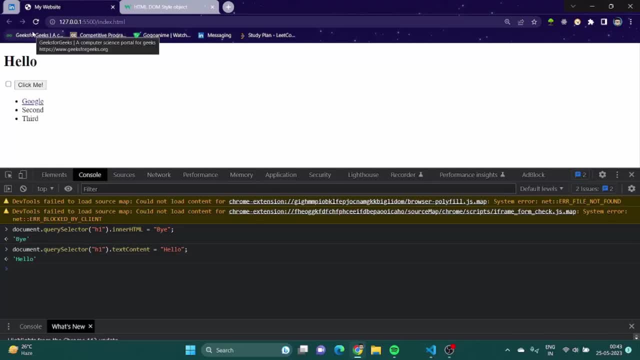 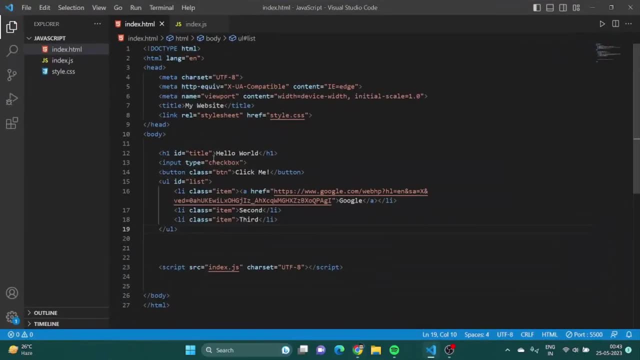 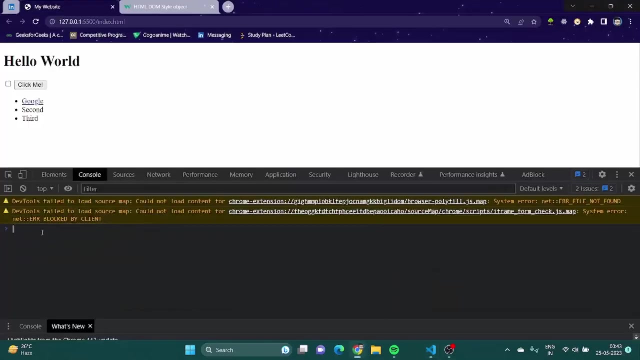 seems similar, but there is a very big difference, i would say, which is suppose i put something wrong. and here again i just put strong: okay, works right. great. now if i go and write document dot query selector, and if i say h1, if i say inner html c, it is giving me the tag name as well, which is hello world. 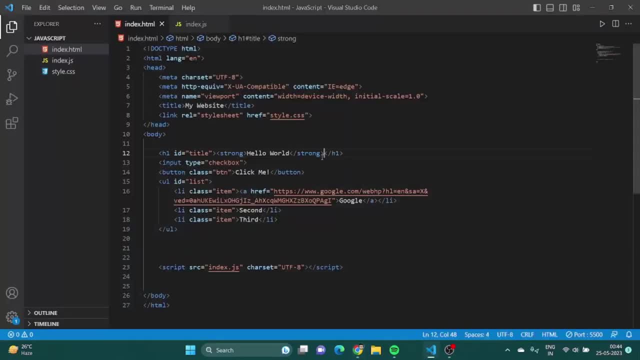 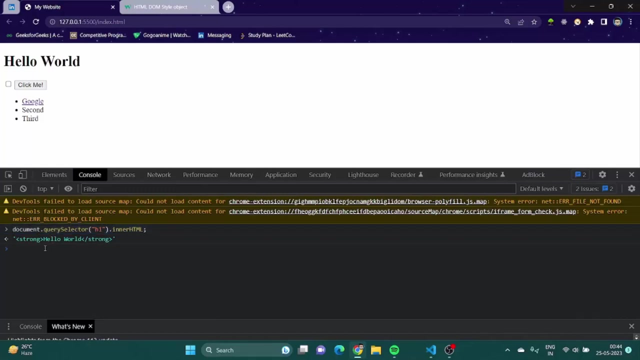 plus strong. so it is basically giving me all the inner html of this tag, which is this whole thing, whereas if i do this part, control c, control v, dot, uh, let's say text content. so just in, tell me this part. okay, that is a very big difference. 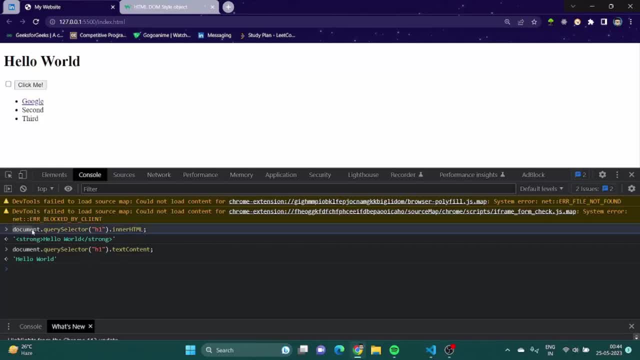 so, using this inner html, you can change the html of it as well. how? let me show it. i'll just copy it and i'll just paste it and i'll say, uh, let's say em and let's say hello. only see, you can change the uh html properties of it as well. 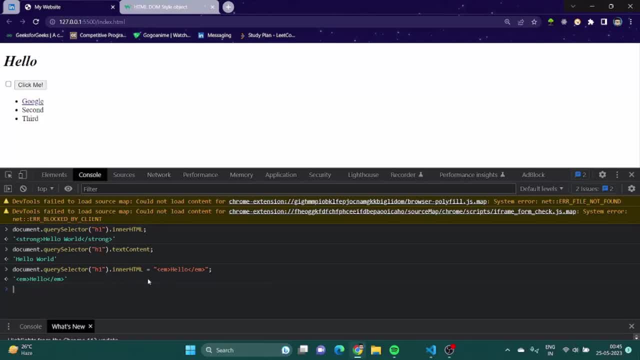 okay, so that is another big uh plus point of inner html. great, so now that we have seen how you can manipulate the style and the text of an html element, the last thing that is left is to how to change the attribute of an html element. okay, so. 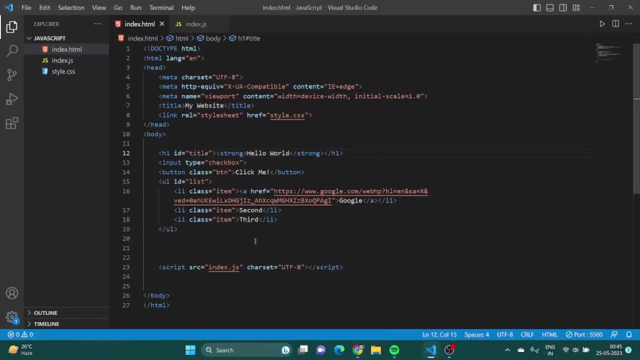 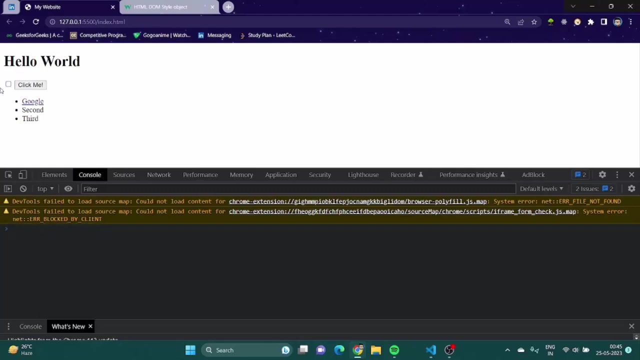 what are attributes? attributes are basically all this um orange thing you are seeing, like href is an attribute, okay. this item is an attribute. this checkbox is an attribute, okay, great. now how you can, you know, tap into any elements attribute. let's see that. i'll just say query select. 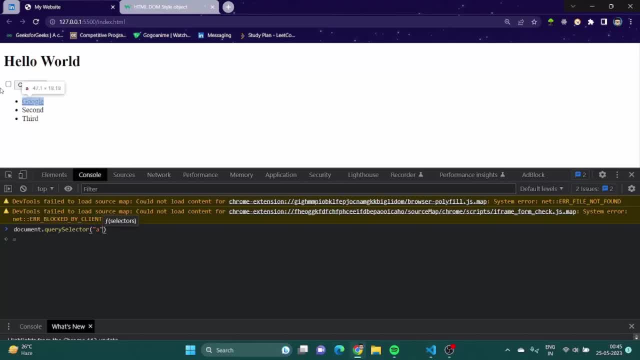 the, and here i'll say a, and here i'll try to find the attributes of it, which is: you know, it only has one attribute, so length is one, which is href, href. you can open it and here you can find everything, like. there's a lot of details which you don't want to get into now. if you want to get a,